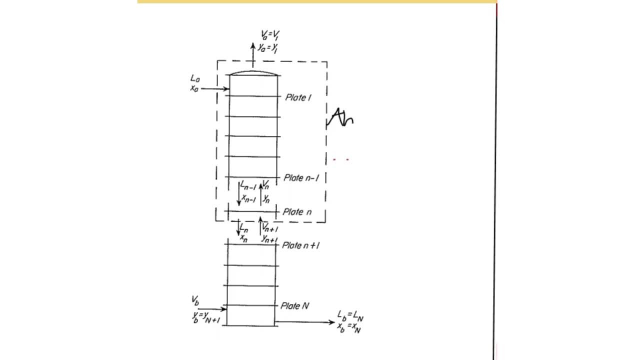 What is absorption and stripping? Absorption and stripping? I will explain everything from the diagram. you are seeing This very diagram. But before coming to the explanation, I would like to explain what absorption and stripping is. Absorption and stripping are separation processes by which we separate two materials. 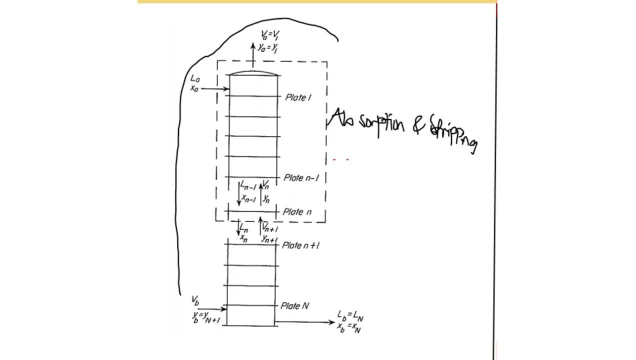 What did I say? Two materials of different phases, And the phases are vapor and liquid. So therefore it's a VL separation, Vapor separation or gas, then a liquid inside a separation column. This diagram I've just drawn is our separation column. we'll display. 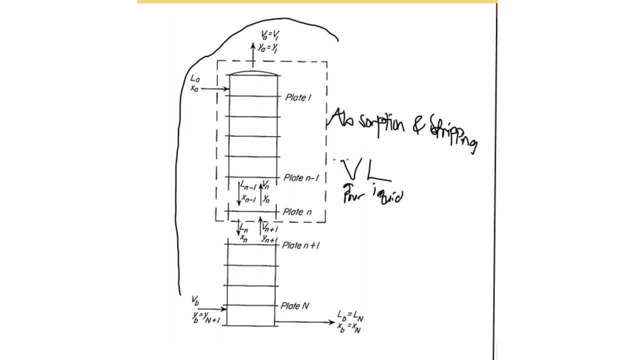 So absorption and stripping are a process whereby two phases, material of two phases- one of the vapor phase and the other of the liquid phase- are flowing inside a separation column counter-currently, so that they mix together and one of the phases receives some materials from the other phase. 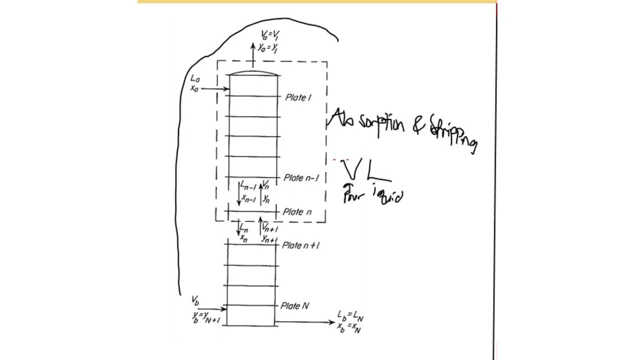 So what is the difference between the two? Absorption is a process whereby the vapor phase, that's the vapor phase, comes into the separation column and then it mixes together with the liquid phase. Therefore, the vapor phase is the one that has the materials we need to remove. 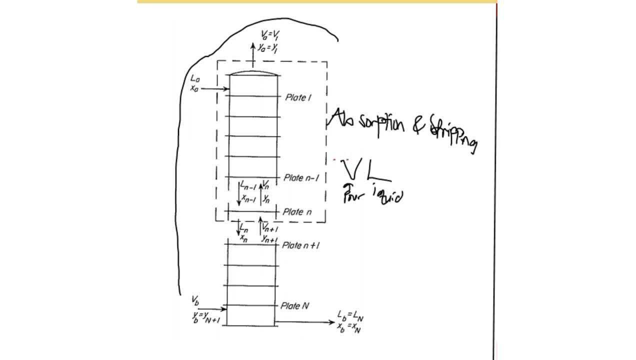 Then the liquid is washed. The liquid will wash that certain substance or certain material from the vapor phase and then the liquid will come out with that material. That means the liquid absorbs the material from the vapor, While stripping is the opposite case, where the liquid is the one that will come with the material we need to strip. 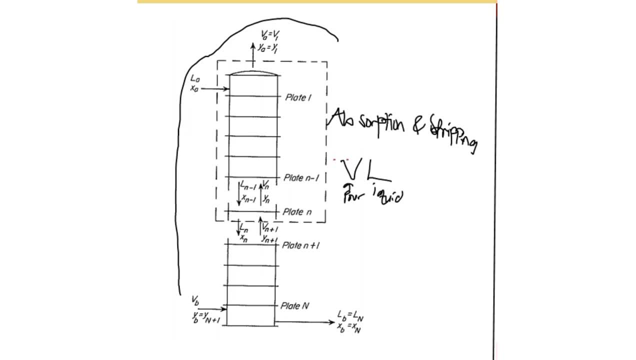 Then the vapor phase will wash away the contents or the substances from the liquid and go away with that substances. That means the vapor stripped out the contents. Vapor stripped out contents from liquid And liquid absorbs contents from the gas And vapor strip. So now I've explained to you what absorption and stripping is. 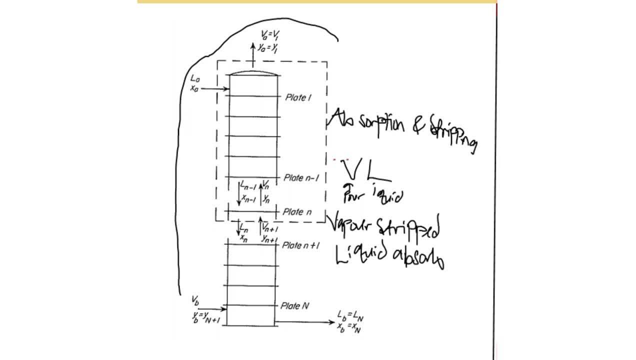 Let's go back to the diagram from the column. You know that when we leave, like a vapor or gas phase, normally in atmosphere, without any container, without anything, what direction do you think would you follow? This is a common sense, Can you think? Will it go to the direction of upward direction or downward direction? If it's vapor or gas, directly it's going to upward direction. You can see it from how you're cooking your food, right. But if it's a liquid- liquid inside a container at a certain space- just remove the container. 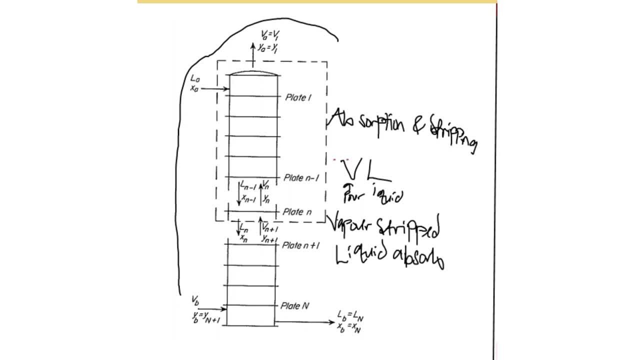 You know that definitely it's coming down because it has a lot of mass and due to gravitational force and the rest. So from this diagram you can see that the diagram have two inlets and two outlets. This one, inlet 1.. 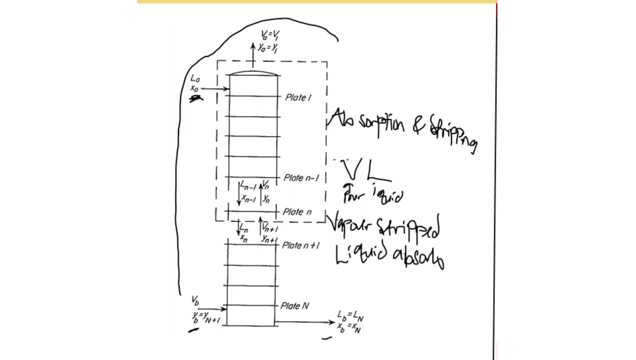 This one, inlet 2.. And this one here, outlet 1.. The other one here, outlet 2.. So where do you think our liquid will come and the vapor will come to, So that they have a good mixture, So that they mix thoroughly, counter-continuously, as I mentioned? 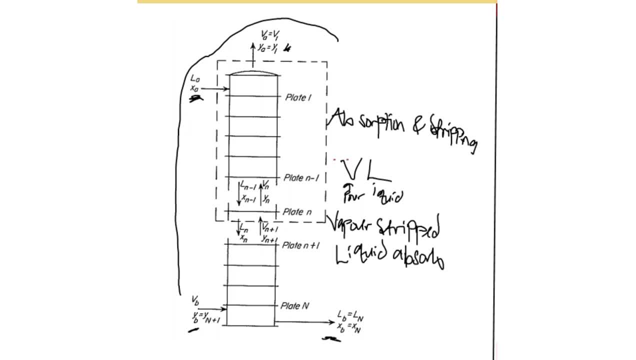 So that we have a good stripping or a good absorption. So since we know the direction of our contents, the vapor is going will go to the upward direction, So it's supposed to enter through the downward entrance, This one here. 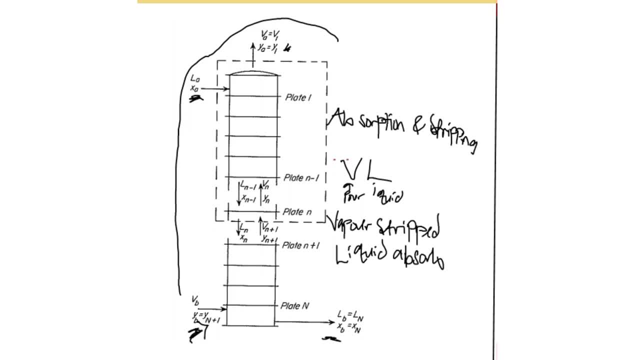 The vapor will enter through this stream and the liquid will enter through this stream As they are coming in. as they are coming in, they will mix thoroughly together, So that we will have good mixture in which one content will receive the other, For example, if it's absorption. 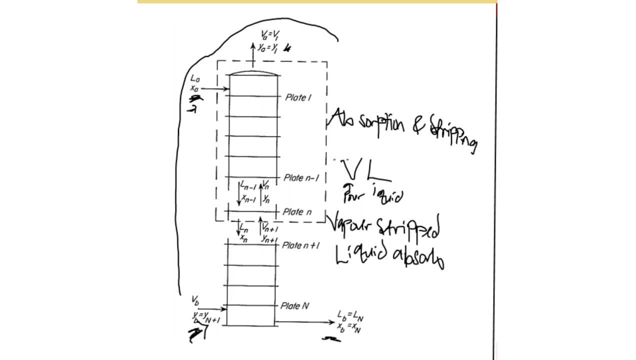 so that the liquid content will receive all the needed contents. So the percentage absorption will absorb it from the gas and it will come through this space, right, The LB, And if it's stripping it's the same thing. The inlet of the gas will be the bottom stream. 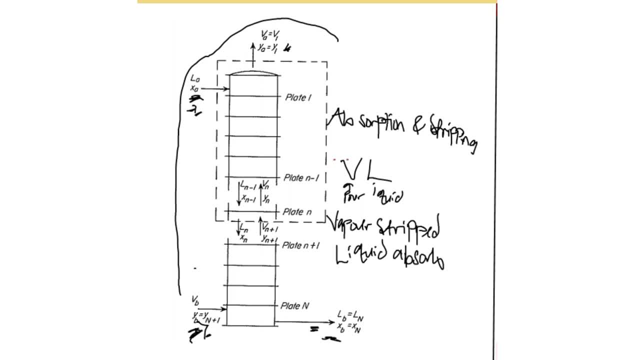 The inlet of the liquid will be the top stream. The outlet of the gas is going to be the top stream. The outlet of the liquid is going to be the bottom stream. I hope you all get me. So what are these notations we are seeing? 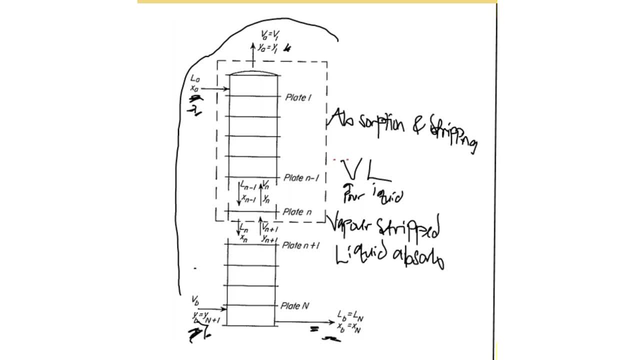 This notation, LAXA, that means for the upward inlet. the inlet of the top stream, is where our liquid is coming. That's why we have the notation of the mass flow as LA, While XA is the mass fraction of our content. 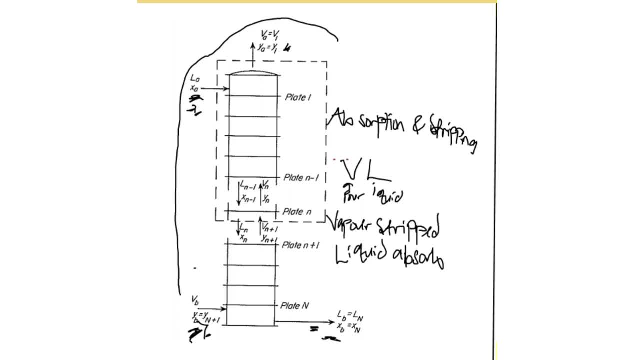 that content needed to be absorbed or stripped, just needed to be removed from the other XA is the content, the mass fraction of that content in our LA phase XB is the mass fraction of the material we are needing in the bottom stream of the liquid. 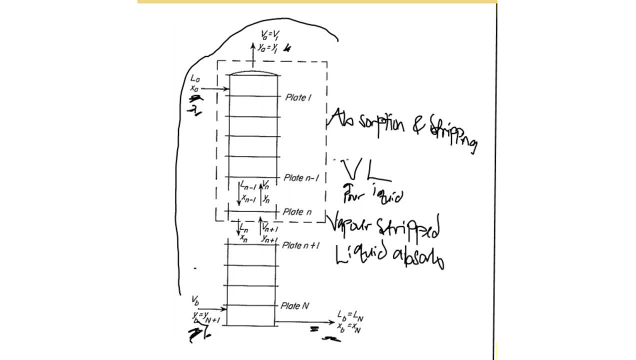 Then YB2 is the mass fraction of our VB, YA is the mass fraction of that content in VA. So you can see that they are opposite. right LA is the inlet of the liquid, but VB is the inlet of the vapor. 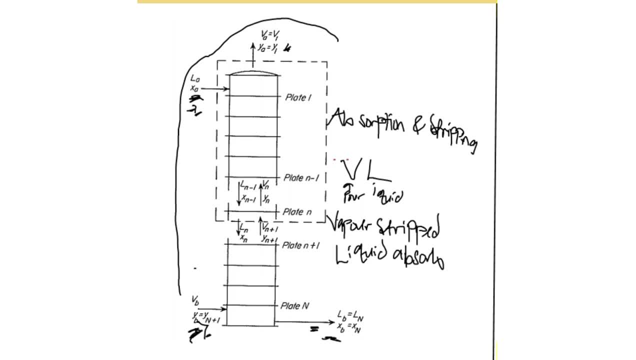 B is for inlet if it's vapor. A is for inlet if it's liquid. So, and you can see these drawings notated by plate 1.. That means the number of plates. It will be plate 1,, 2,, 3, out. 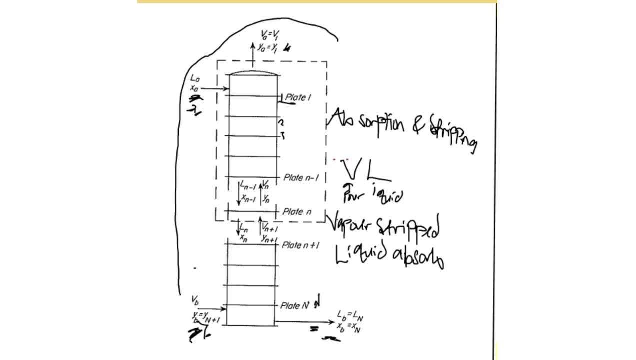 That's the number of plates inside our column. I think you all get this explanation of what is happening: a real stripping and absorption. So, coming back to LA XA, VB, YB, XA is the mass fraction, as I mentioned earlier. 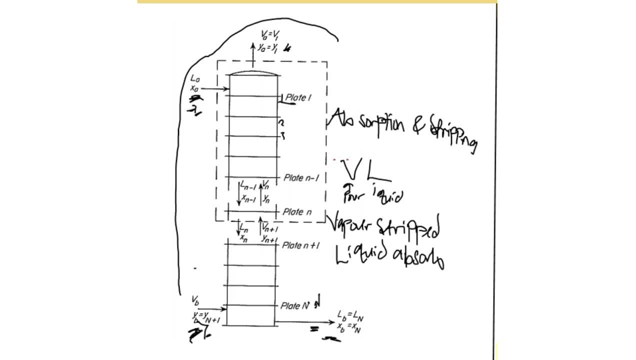 is the mass fraction of the content we are taking our study on. Maybe you can take it as a system, If you don't forget your thermometer, if you don't forget your thermodynamics system surrounding and boundary. So only what we are looking for. 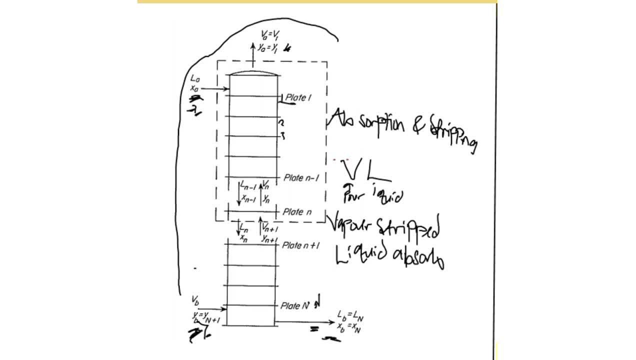 what we are focusing on is the system. So XA is our system in liquid phase. So YB will not be the mass fraction of the other phase or the other material. It will be that same, the mass fraction of that same material. 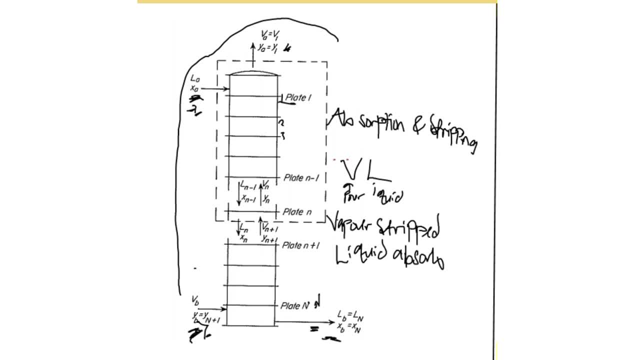 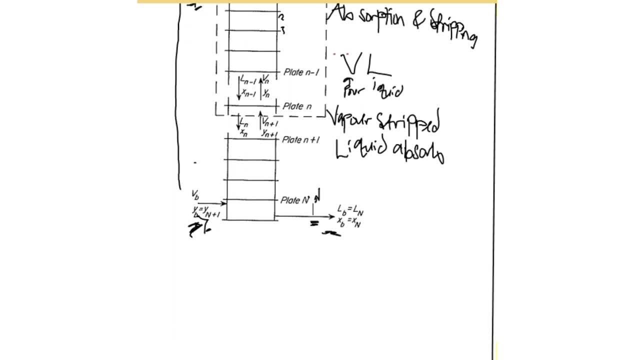 but because it's in Y direction, that's why we will name it. Because it's in Y direction, that's why we call it as Y. I mean because it's in V4 phase. that's why we are going to call it as Y. 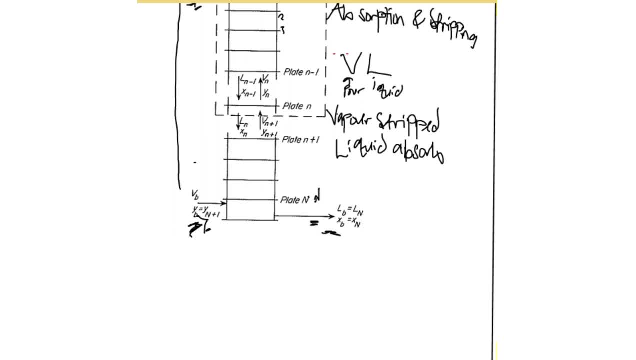 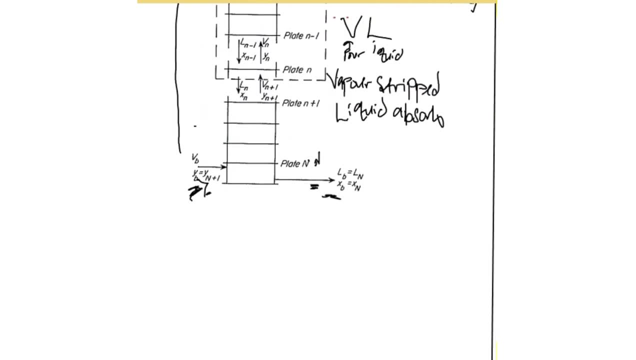 the mass fraction. So now I explain what stripping is, what absorption is, and I explain how they happens, how they go in and how they mix and how they go out of the column. So now, how do we solve problem of stripping and absorption?